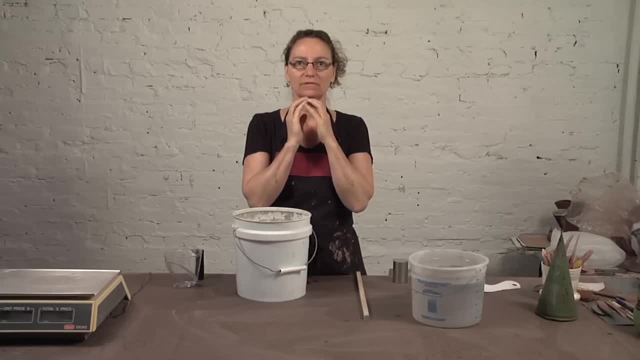 to look like a skin rather than you know something highly reflective, And so I really just didn't. I didn't have quite enough knowledge to get to the point where I had a satin clear that was consistent, And so Carla came and she worked with me and 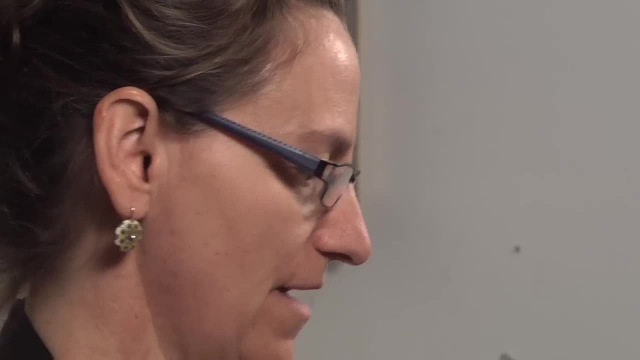 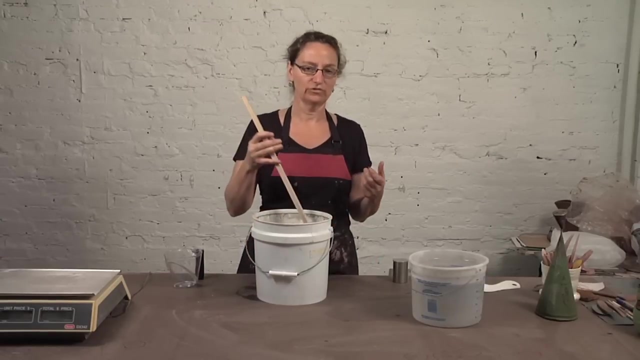 we developed this, this satin clear glaze that we're going to use. now. The thing about working with an engineer is they really know what they're doing And, as far as like the tools that are used in industry versus the tools that are used in potter's studios are, 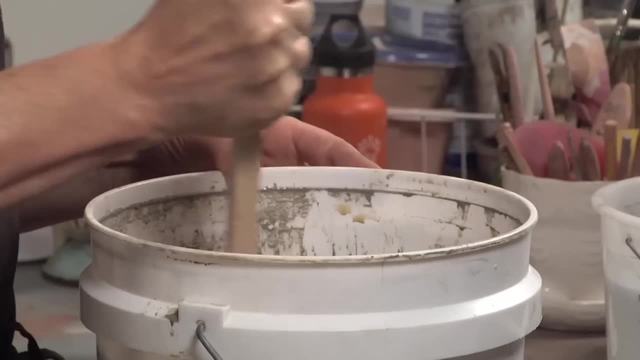 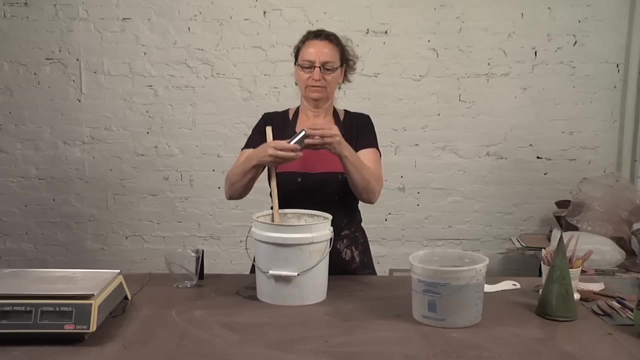 different and you know, there's no reason why we can't have some more overlap than we currently have. One of the things that Carla introduced me to is a density cup, This little thing. it holds exactly a hundred centimeters. Speaker 1. 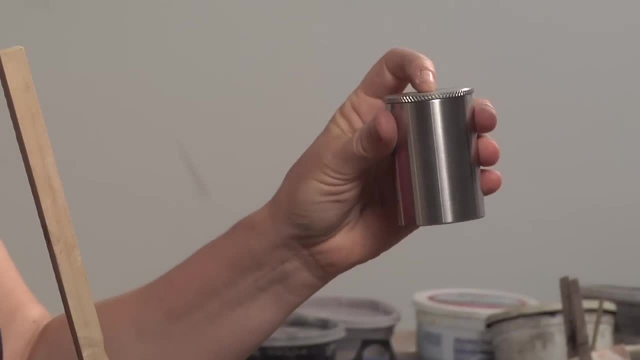 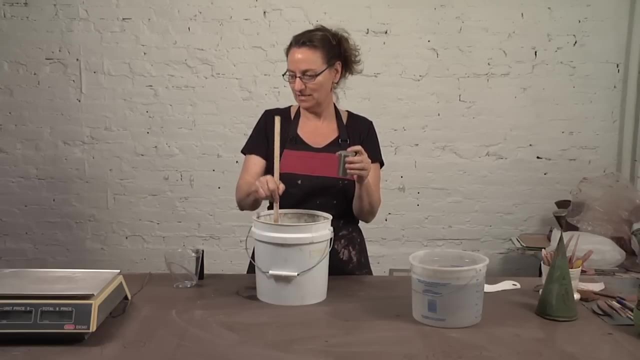 of cc's of fluid and it weighs 200 grams. It measures density to within, well, to whatever your scale will measure. In this case, we're using an old butcher scale which measures out to a hundredth of a decimal place. I have an Ohas scale at home which does the same. 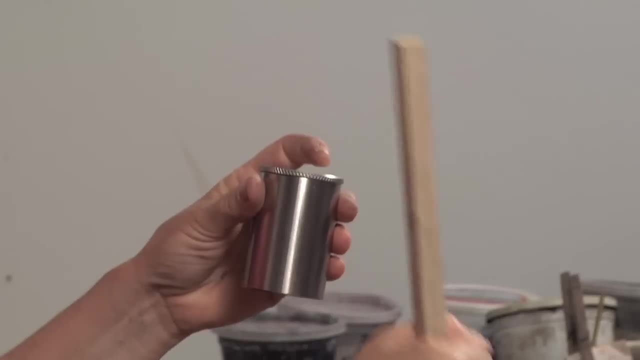 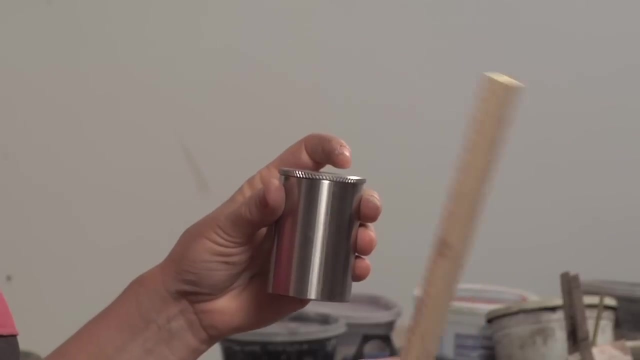 thing She also- you know that was another Carla addition- was to get me to use a digital scale instead of a triple beam scale. The triple beam scale works perfectly well. It just takes a lot longer to wait for that scale to. you know, balance out. 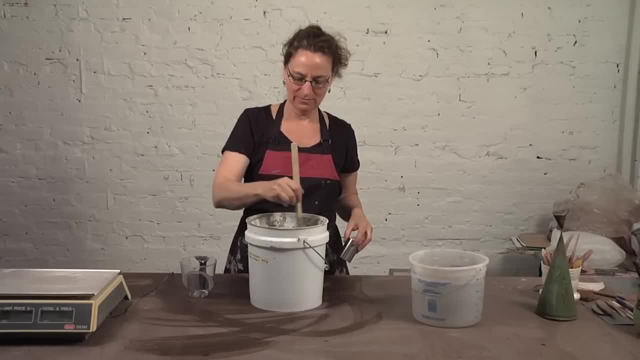 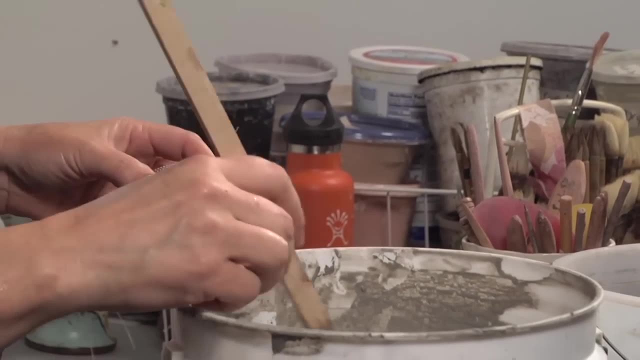 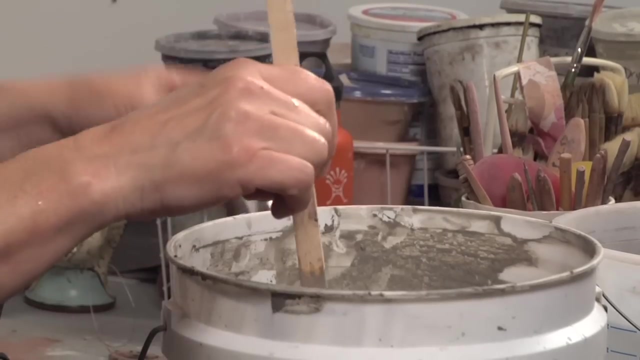 So all you have to do is mix In order to get consistent results from your kiln. if you can measure density, you've reduced one of your variable, one of a very important variable. You know, some glazes are more forgiving than others. You know, potters are typically. 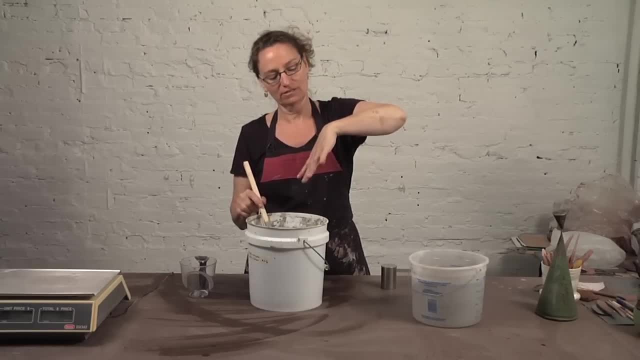 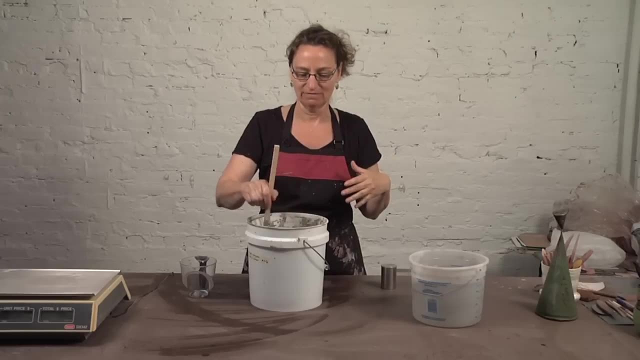 they'll put their hand in and they'll watch it slake off and just say, you know, they can see their skin or they can't see their skin. whatever their measurement is visually, they can visually kind of calibrate how thick or thin their glaze should be. What I've learned 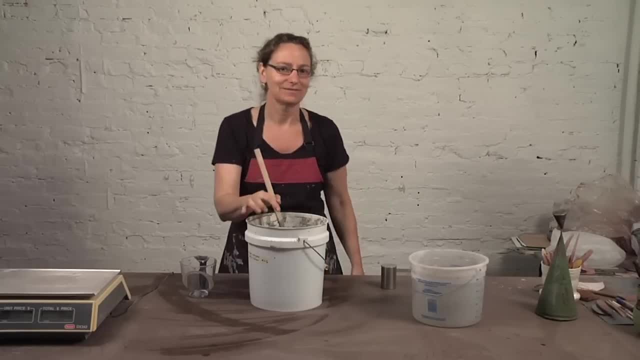 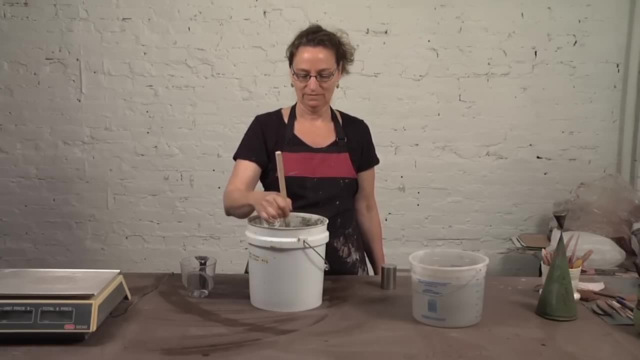 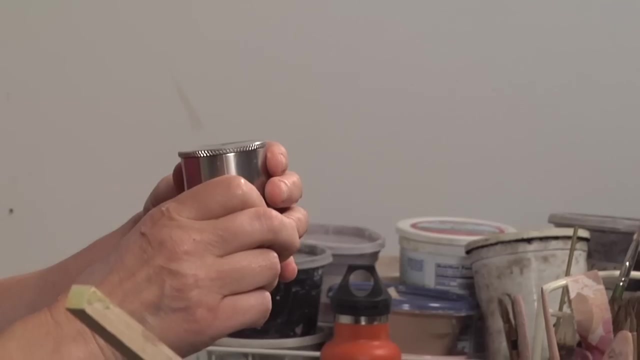 through working with an engineer is that it's not about thickness, it's about density. A glaze can appear quite thick depending on what's in it and and not be very dense, and vice versa. So the cool thing is that I now have this density cup. 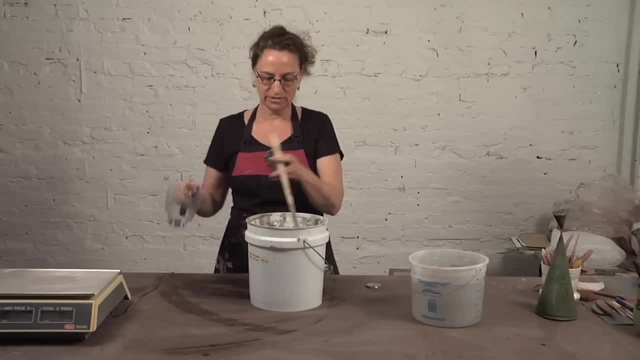 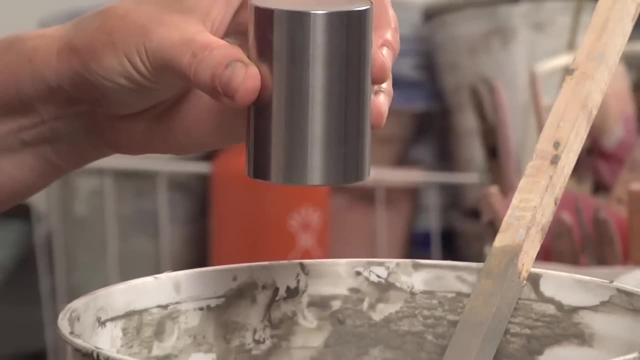 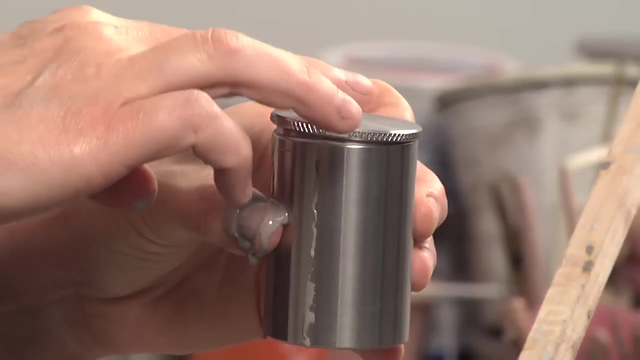 which is used in industry, and you can too. So what you do is make sure your glaze is well stirred, fill your density cup past that meniscus point, put your lid on and the excess is going to come out. See how I just made that little. 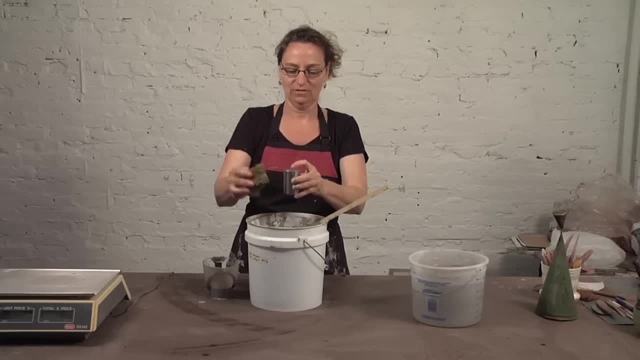 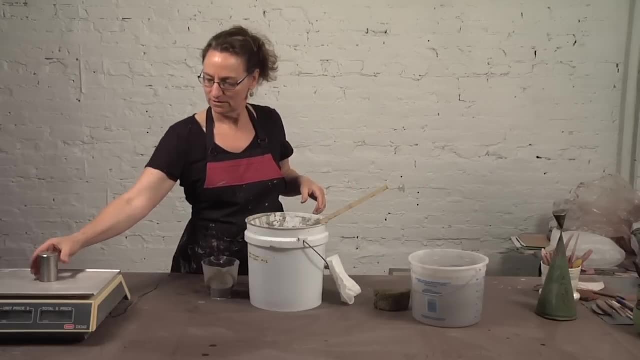 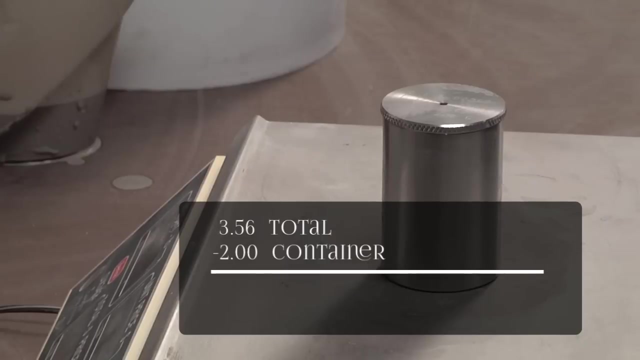 fountain. Perfect amount: exactly a hundred cc's, no more, no less. Once you've got the excess wiped off, you put it on your digital scale. so my reading is 356.. The cup weighs 200.. Water: a hundred cc's of water weighs a hundred grams. 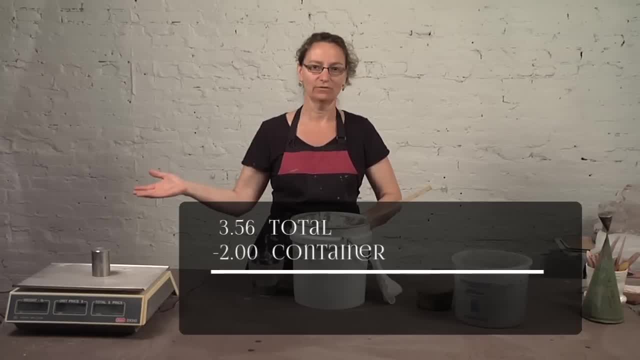 and so the extra, the overage, so 1.0 density is water. So anything over that is what the density of the glaze is. So I'm going for 1.44, and right now I have 1.56.. So all I have to do 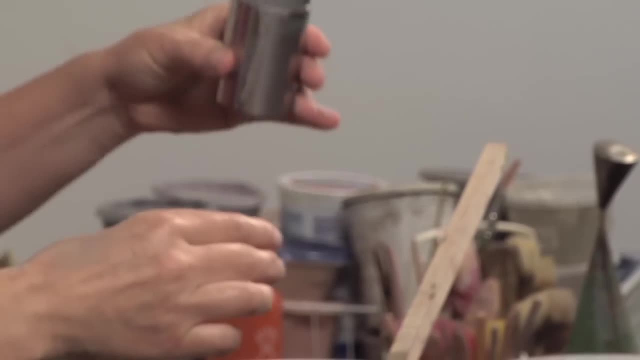 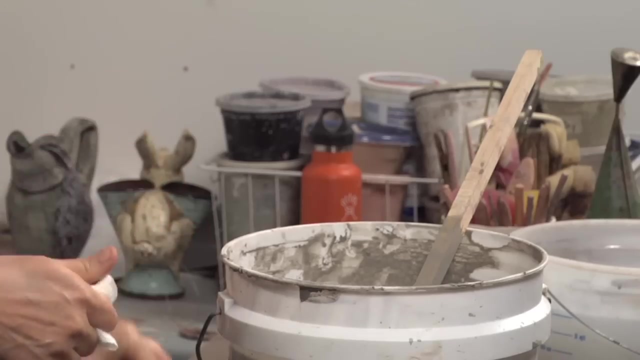 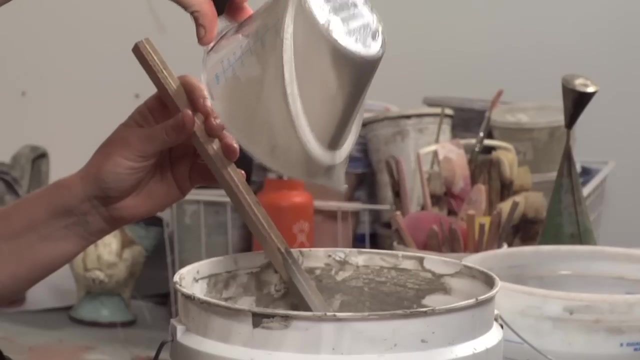 is: dump it out, wash it out, dry it out and then I'm done. Dry it out because you want to use every little bit of the capacity. Add some water, that's the extra glaze. You know, and it's an educated guess, how much is enough water? 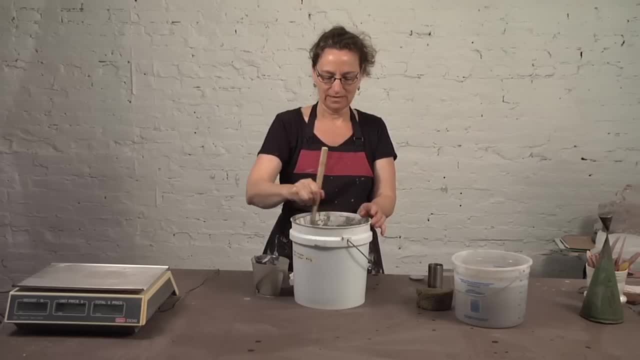 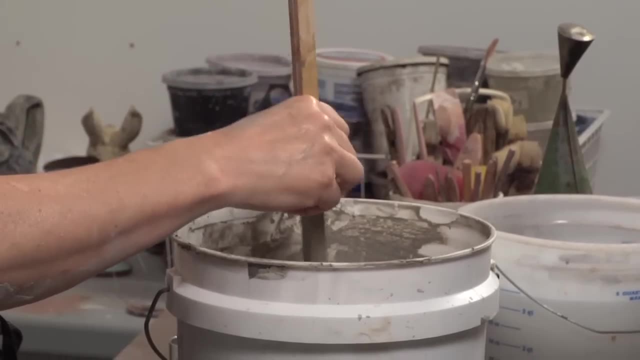 You might be saying to yourself, I don't need that, I don't need that much accuracy, and you might not based on your glazes, but for the production potter who's got dinnerware going and it's a blue glaze, density matters. 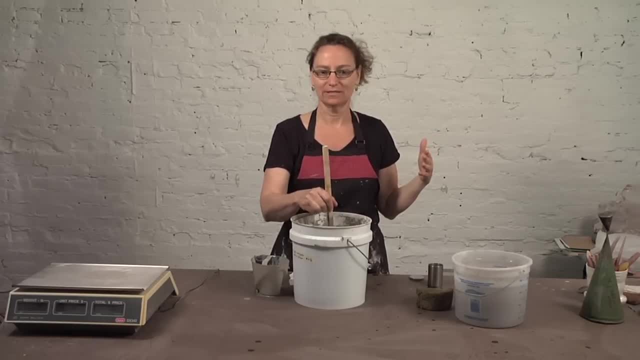 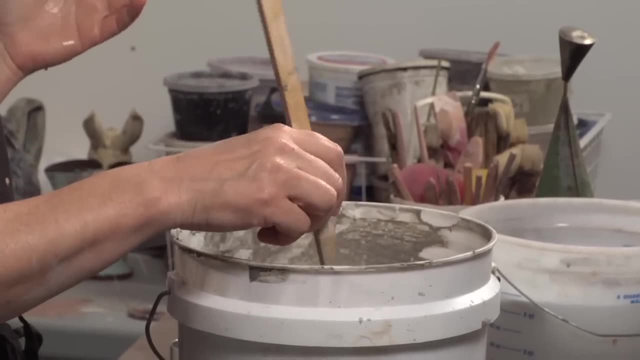 Like, the shade of blue you're going to get is going to be somewhat dependent on density. So you've been making this dinnerware, say, for a couple years and all of a sudden somebody calls you and says: oh shoot, you know I broke a plate. Can you remake me that plate? 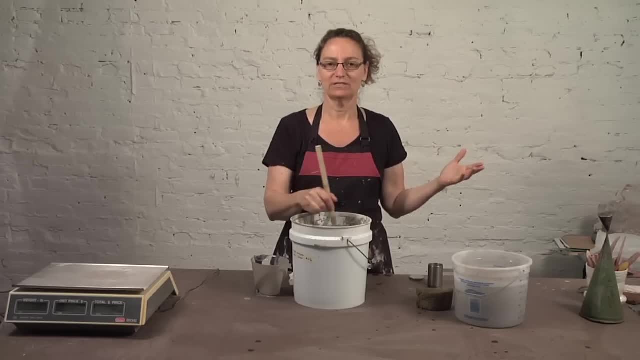 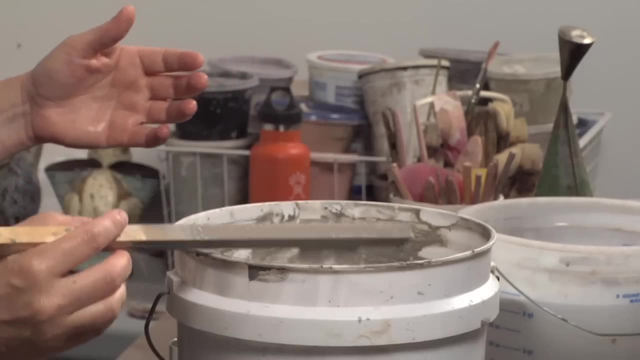 And so you're like no problem. Well, if you can't, if you didn't measure density, it's going to come out likely a different shade than the rest of her set. Some people don't care, but if you do, then maybe this tool will help assist you. 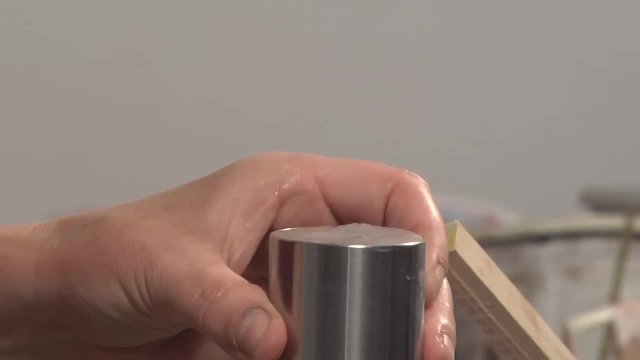 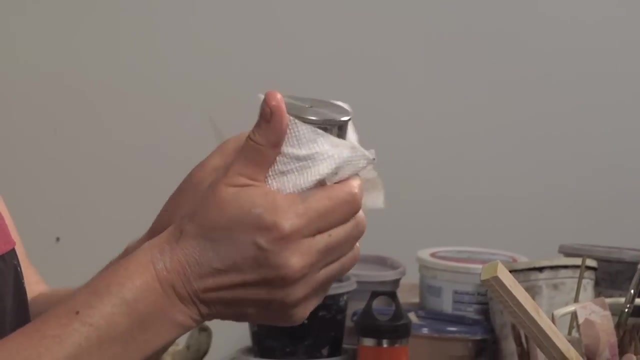 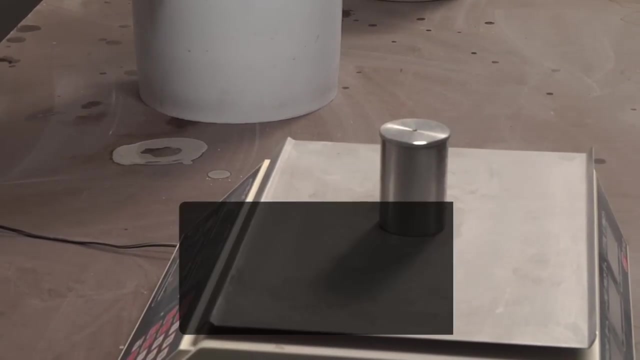 So, once again, you're going to want to make sure that you've got the right density for your glaze. So you're going to want to make sure that you've got the right density for your glaze, And now it should be closer to 344, 1.44 density. 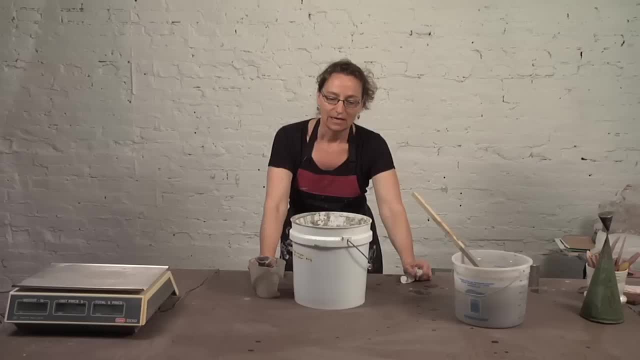 And we nailed it. So now it's good to go. And so it was only through trial and error that I realized that 1.44 was the optimal density for my glaze. If my glaze is more dense, aka thicker, then it's good to go. 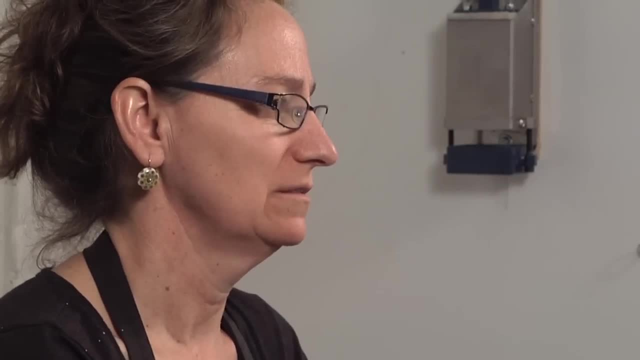 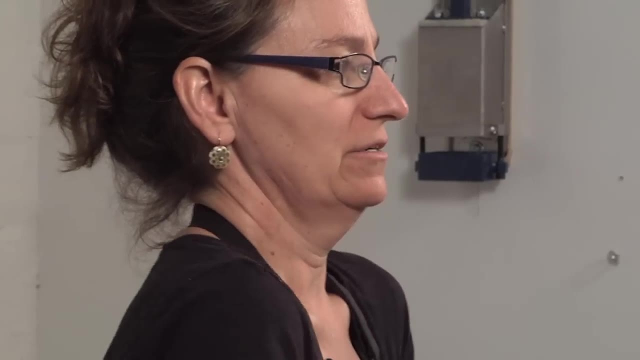 If my glaze is more thicker then it gets shiny. You know it's too much material. And if it's too thin, if it gets to be more like a wash, then it doesn't really have enough material to give it that magical satiny crystalline surface. 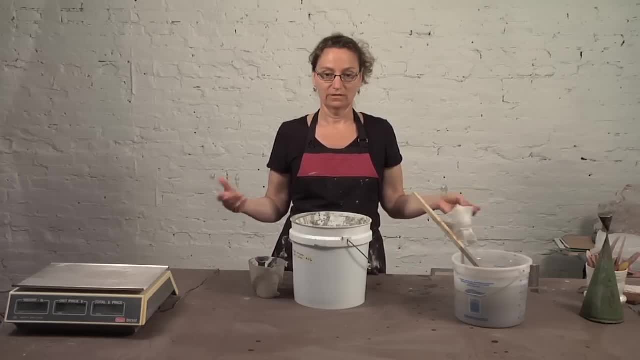 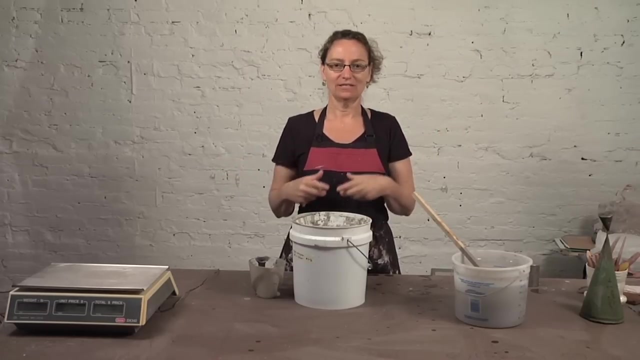 Your glaze when you're not. you know if you're not using this Naples Wagner Satin Clear, you just have to play around with it. You know from your hand-dipping or whatever way you're measuring what's like if my glaze is good to go that, measure the density, throw the kiln in. 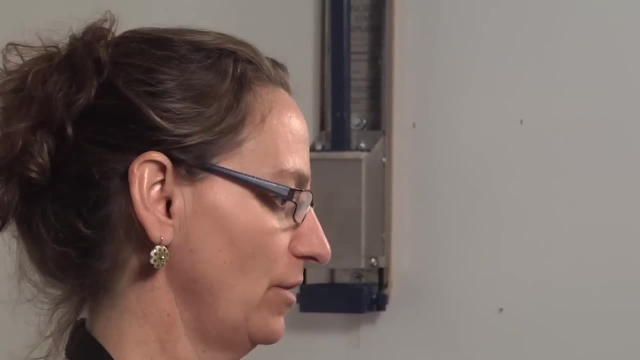 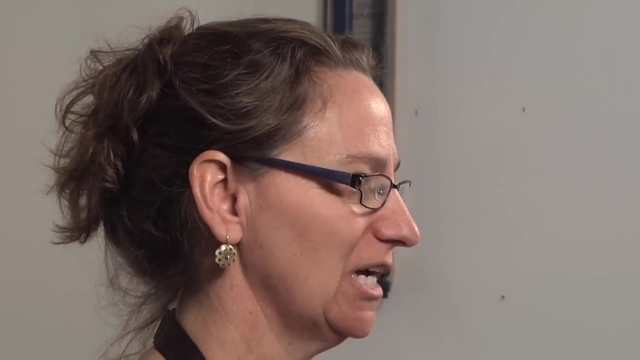 get the kiln out and say: I nailed it, I love the glaze, just like that. Well, you recorded the density, so now you know what your measurement is. You get the kiln out and it's like ugh, it got washy. The color looks washy. 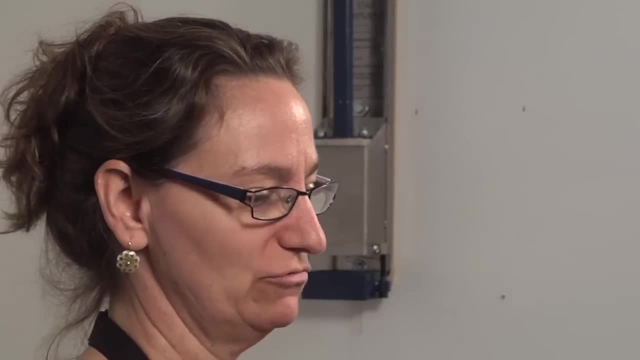 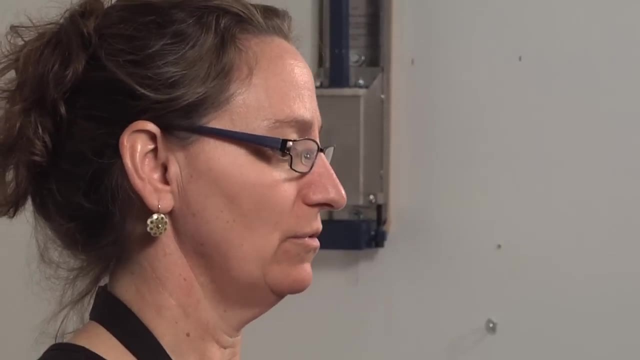 Well, it wasn't dense enough. Now you can test. You can actually, you know, just run a test kiln with varying degrees of density and see which one you like the best, And then put it on a whole body of work, a whole kiln, load of work. 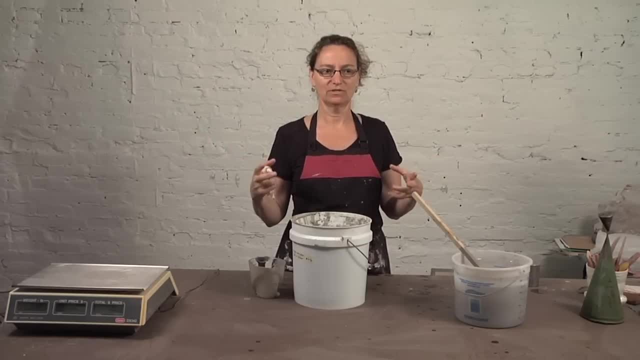 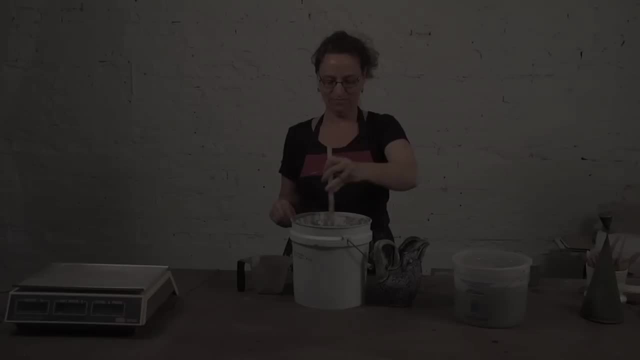 and then you really get a bigger picture. You know, just doing tests is great to start, but then you have to apply it to a larger expanse of work to really get to see the potential of it. Because my glaze does settle. it's got some frit in it which likes to settle out. 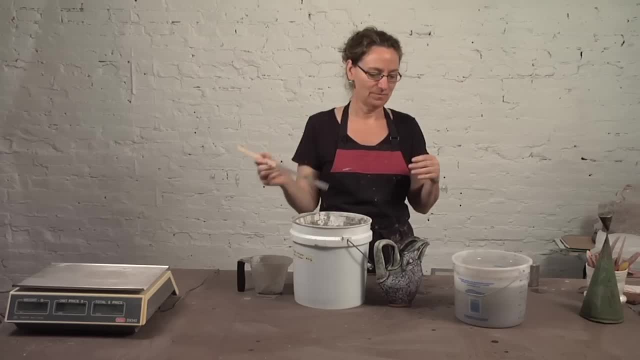 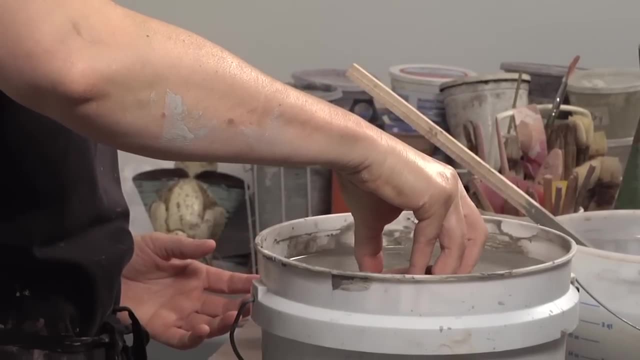 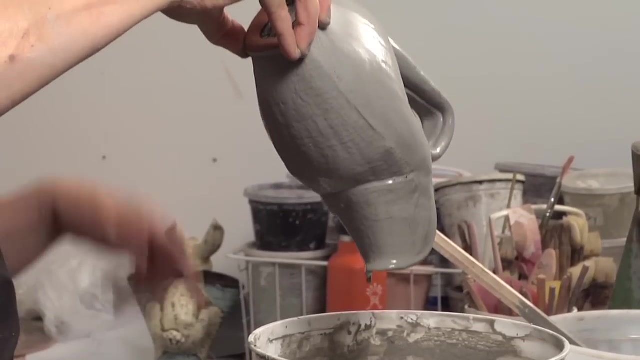 I stir it before I dip things. make sure all my particles are in suspension, And I'll take a pot like this: hold it from its foot, dip it right up into the foot and out. The consistency of your application is important. If I put it in and held it there for a few seconds, it would be absorbing, absorbing, absorbing more material. 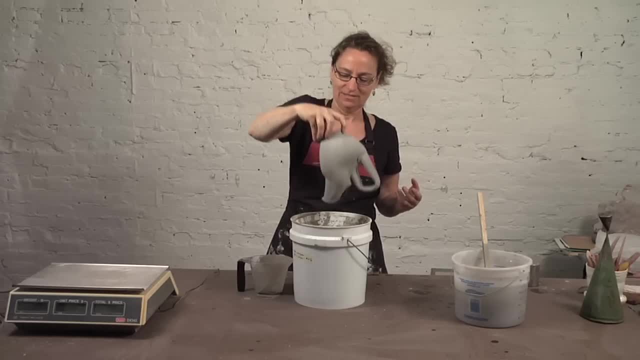 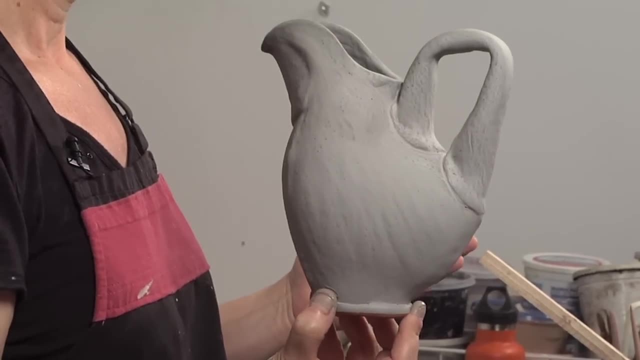 So you can measure your density, and that's helpful. but you could also say: if your application processes are consistent, then your results will be consistent. If one day you're dipping, another day you're pouring, or some objects you pour and some objects you dip, 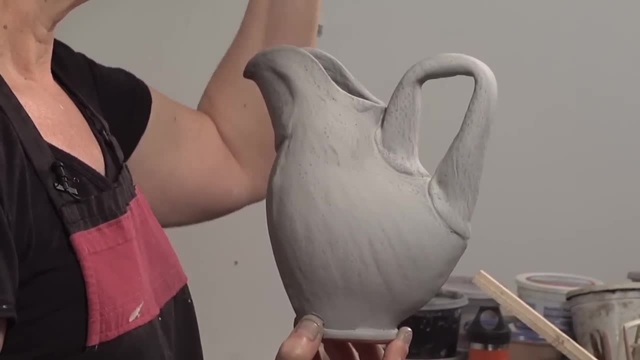 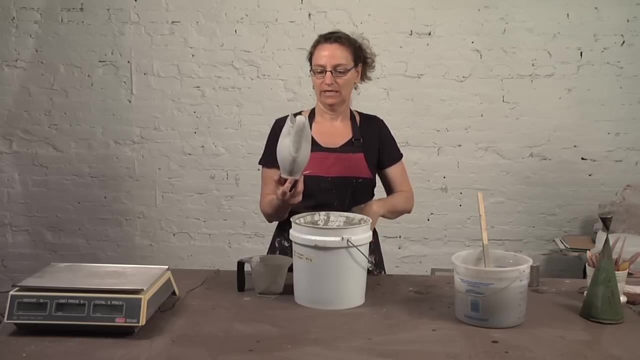 you'll just have to sort of play around with that And learn what the optimal kind of approach is for your work. For me, there are some things that I can't dip, that I have to pour, And so in my case, when I'm pouring those things, it's not just like done. 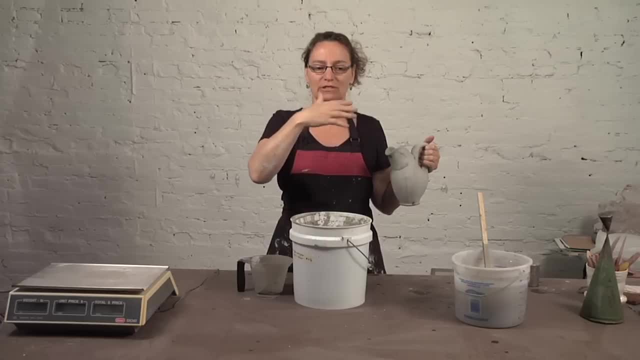 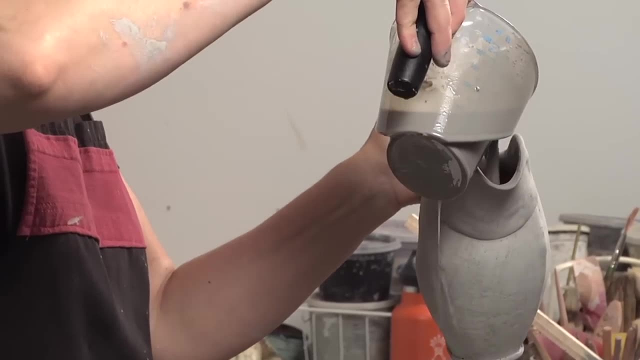 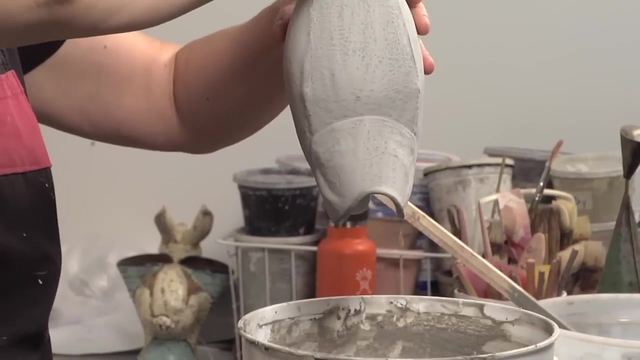 it's like slow pour, so that it has enough time to accumulate enough material. And so then, to get the interior of this, just use a measuring cup, any kind of little pitcher pour, Just do that. I turned it as I poured it out, so that it would coat the whole rim. 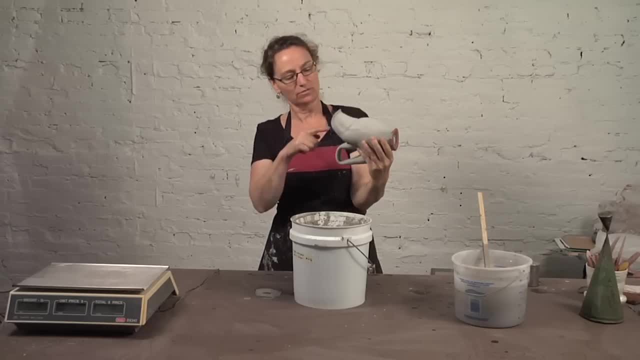 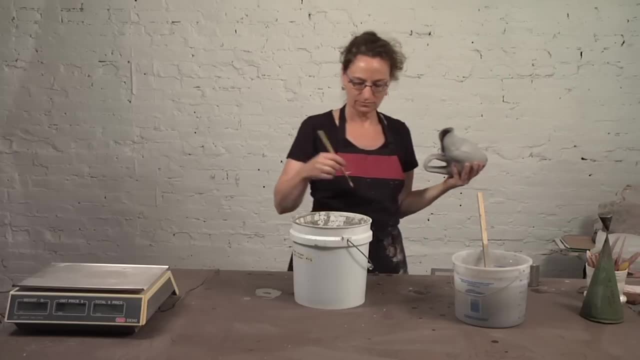 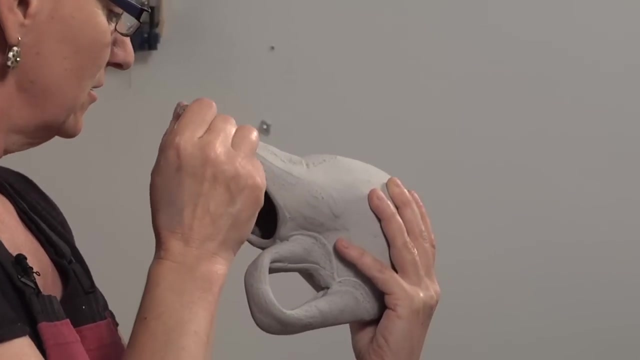 And that worked pretty well. There's one patch in here that's bare clay, So I'll just take a brush, grab some glaze And you know, this is just clear glaze over raw clay. So you know, if it's a little thicker or thinner, it don't really matter. 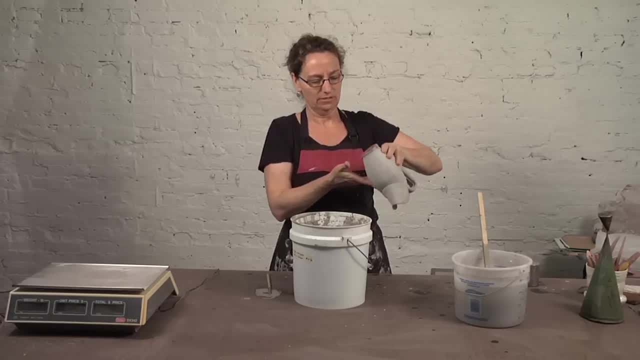 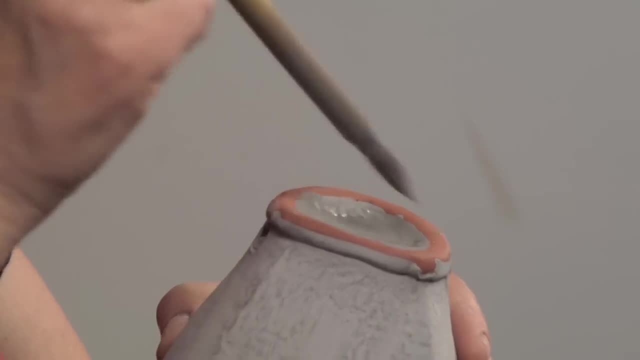 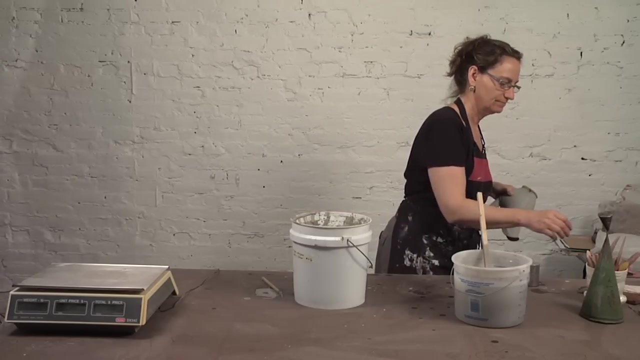 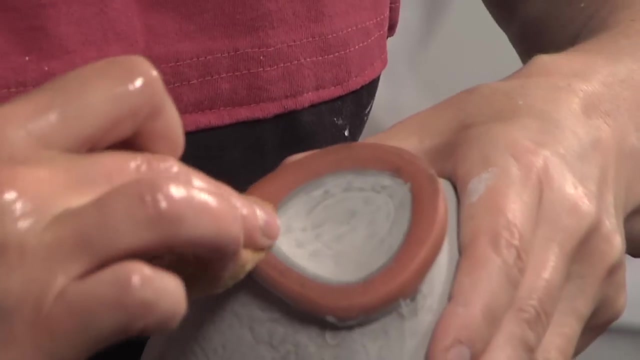 And then, of course, pour it in. That's the first we need to do. I am more trying to get a consistent application than worrying about whether I get it on the foot or not, Because I can take my sponge and just wipe that off. 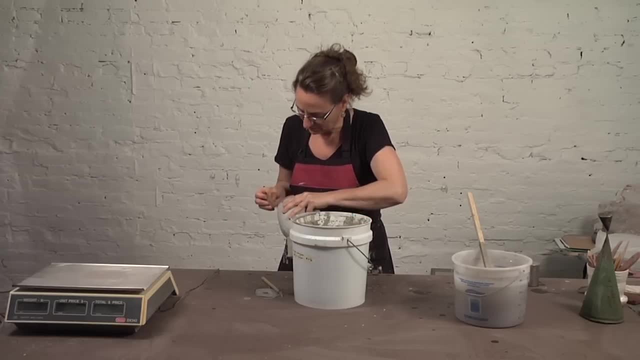 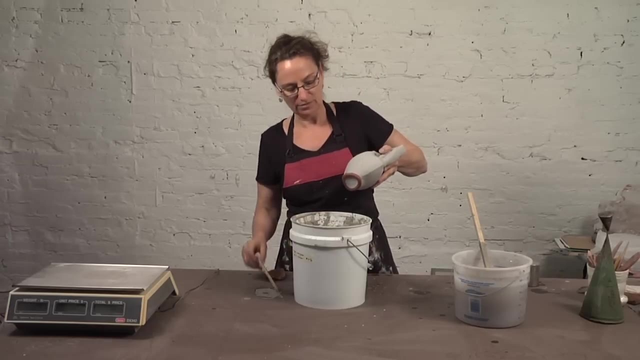 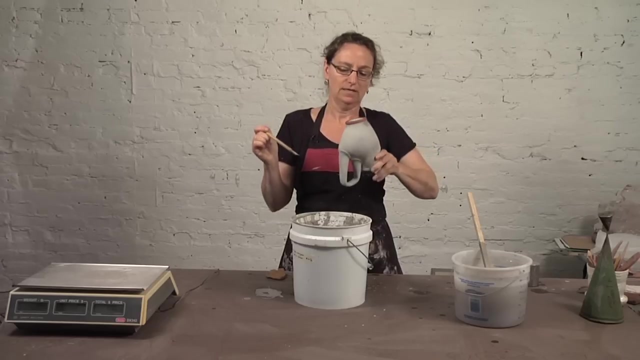 I bothered leaving a nice terracotta foot, so I'm going to take the glaze off of it So that it can show, And the little places where my fingerprints are dab it with a bit of glaze And that pot is ready to go in the kiln. 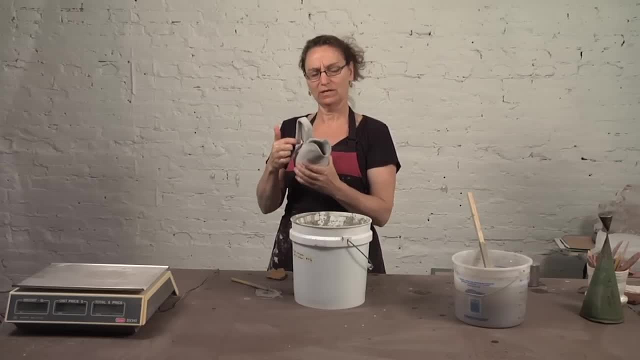 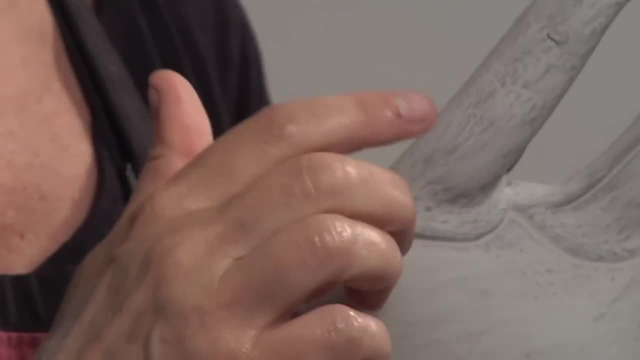 As far as you know, there was a small opening that the handle left. Sometimes that opening is larger, In which case the handle will fill up with glaze, And then, when you go to dump it, it all comes gushing out there. 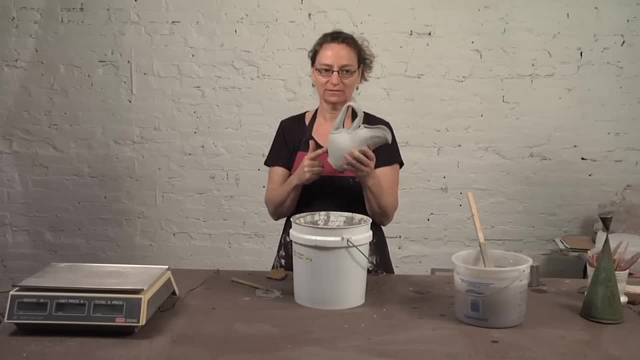 Which can leave an interesting mark. You know, it's just a thicker place, So the glaze goes from satin to a little line of clear and then satin, Which I don't really mind. But if you wanted to keep that from happening, I would just take, you know, the sponge.